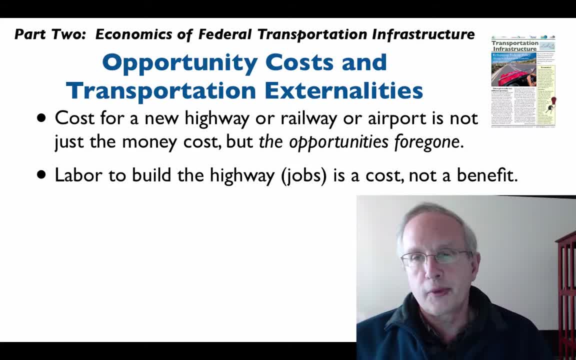 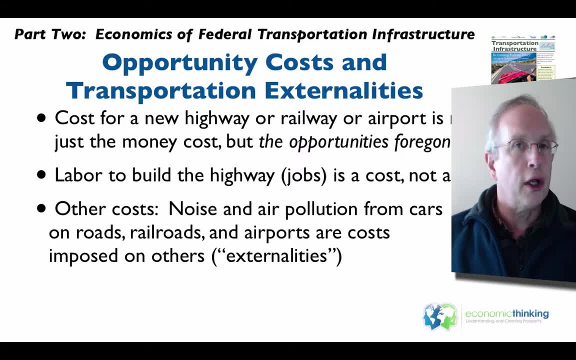 the job is not the benefit, It's what is created with the job. that's the benefit. It's worth mentioning other economic aspects of transportation of roads is that the noise and the air pollution from cars on roads, railroads, airports are costs that are imposed. 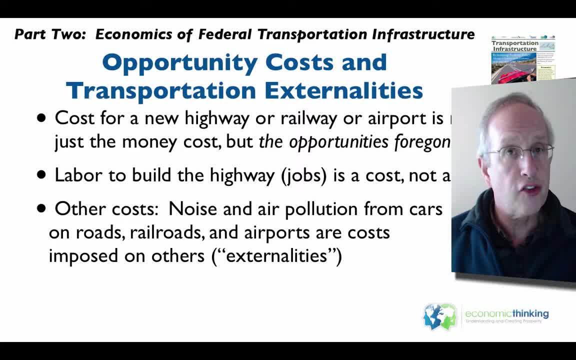 on others. These are externalities costs that are often not compensated. So when a new highway goes in and there's a roar of traffic on that highway, there's a roar of traffic on that highway. the people that have to put up with that noise should be. 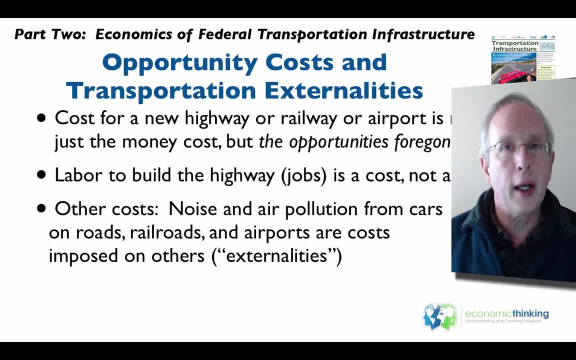 compensated. Now maybe there's some compensation being close to a highway and so forth in terms of value for commercial real estate. But in general you want a system where air pollution, noise pollution, other costs from business enterprises are compensated, They're not forced. 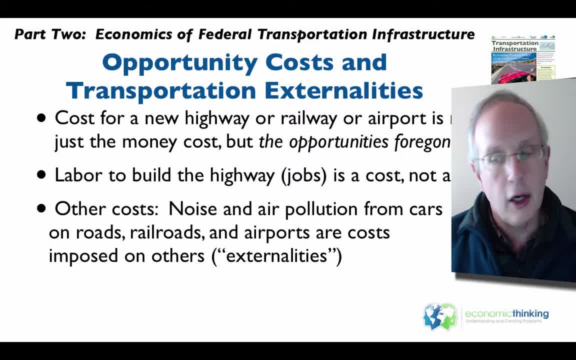 upon people against their will. But again, externality is a little tricky concept. I mean, anybody that lives near a house full of kids has the opportunity to do that. I mean anybody that lives near a house full of kids has the opportunity to do that. And 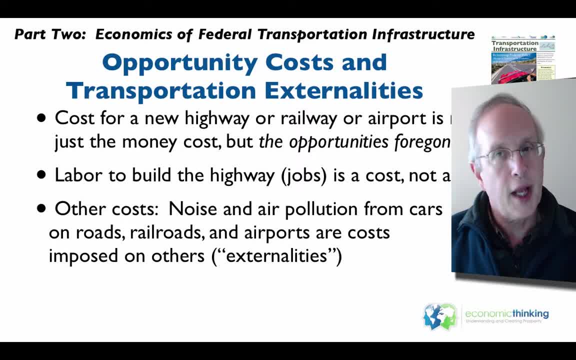 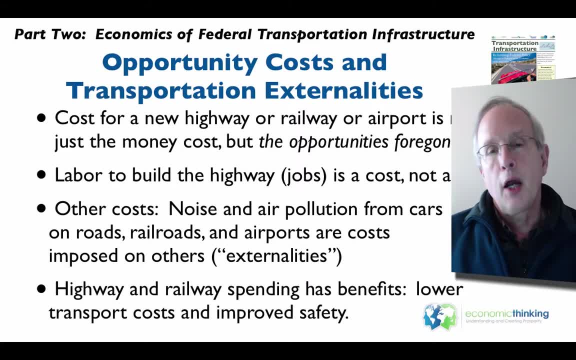 the externality, the kids screaming and making noise So you can't have a blanket. all noise gets compensated, But I just mentioned that as economic aspects of highways, Highways and railway, spending has benefits, of course, and the key benefits are lowering. 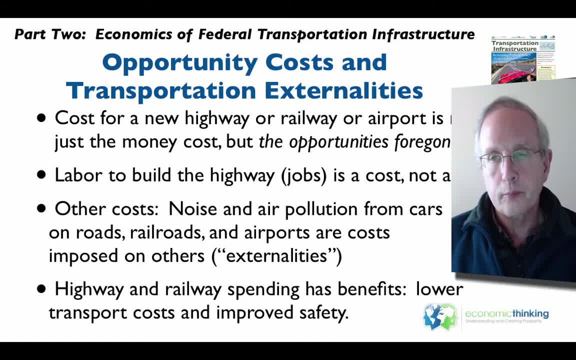 transportation costs as well as improved safety. So new railways that can carry oil across the country or coal or coal slurry. those rail lines allow energy to get from where it's dug out of the ground or piped out of the ground to people that use it, whether 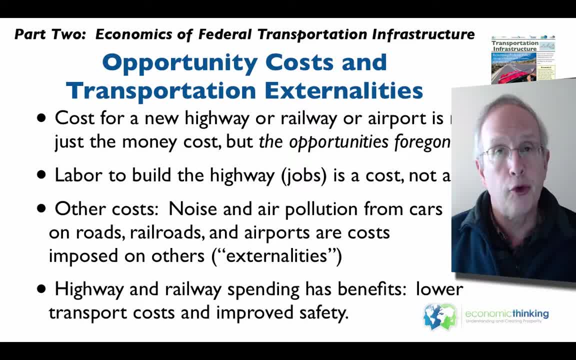 that's a railroad, or whether it's shipped in trucks, or whether it's through a pipeline. Those are all substitutable transportation technologies. The benefit is lower energy costs, companies being able to maneuver to send oil and coal where it's needed most. For a company, again, being able to get parts delivered more quickly, less expensively, is 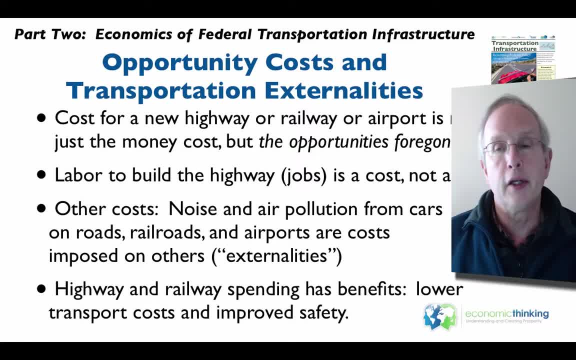 a benefit to the company. It allows US companies to be able to get parts delivered more quickly, less expensively. It allows US companies to be more competitive with those overseas. Improved safety is a key issue for this topic And I know in the public school world a lot. 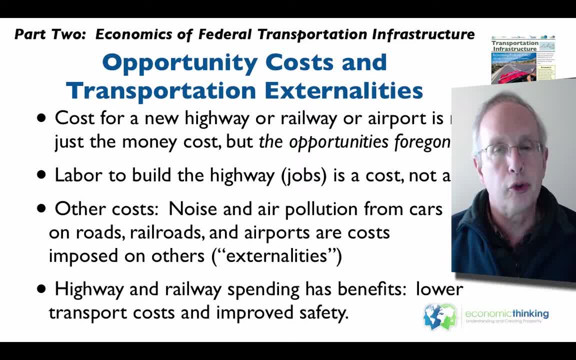 of students were excited about cases that involve improving safety. Lots of people die on the highways. You can look up the numbers. It's a huge tragedy. There's all sorts of commotion about killing with guns and mass murders, but far more people. 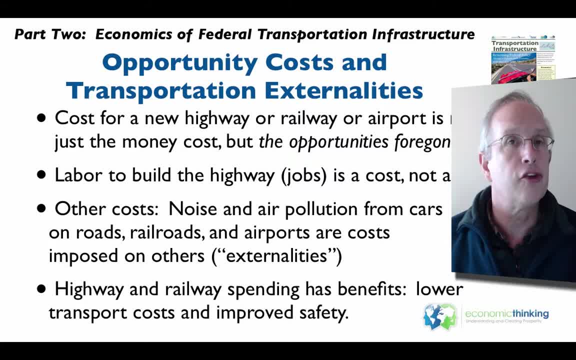 die on highways And that's because the highways aren't designed as safely as they could be. Just dividing highways. I remember in Texas lots of highways that you know. cars are going past each other 40,, 50, 60 miles an hour in the opposite direction. One mistake. 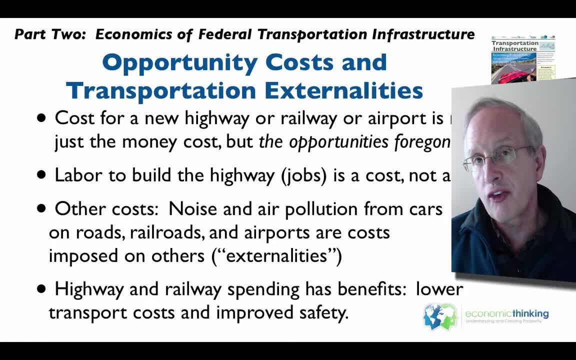 and people are injured or die. A divided highway is much safer, much less likely to have those kinds of accidents. So when you spend money to improve highways, to divide them, to put barriers between the oncoming lanes, that saves lives. Similarly, much less expensively, new white 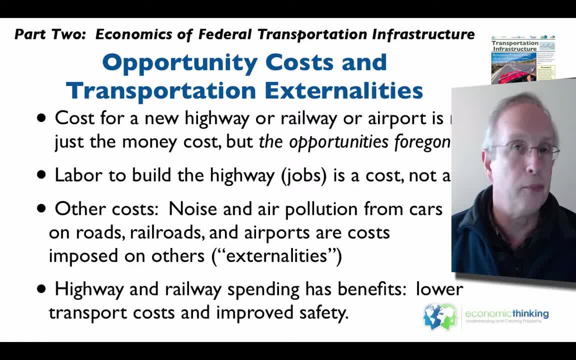 people. we don't have to worry about them going anywhere. It's just a matter of safety for the future of the city. It's also a concern for the nation. It's also a problem for the neighborhoods. If you're driving right there, it probably won't make a difference. It's just a concern for the community. 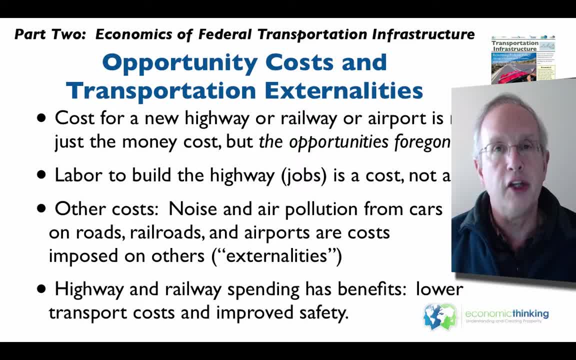 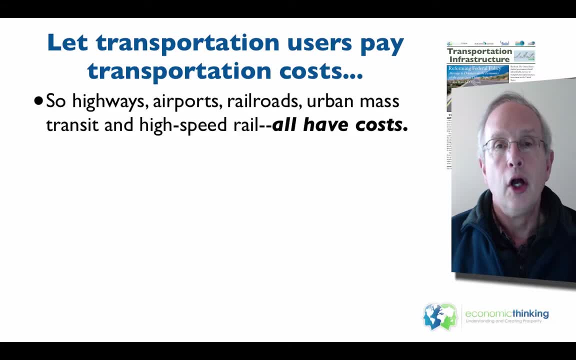 white paint turns out to save lives. It makes it easier to stay in your own side. So there's lots of technologies that can improve highway safety as well as just building and expanding lanes. So one theme in the way economists look at transportation issues is to have highways. 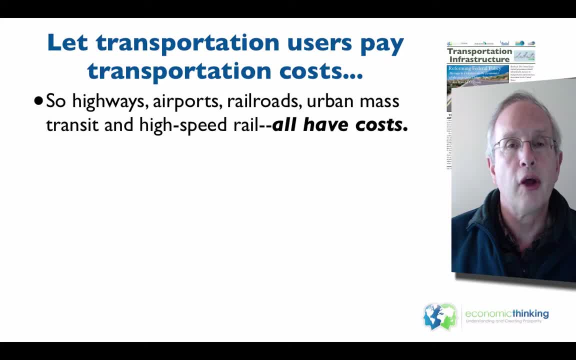 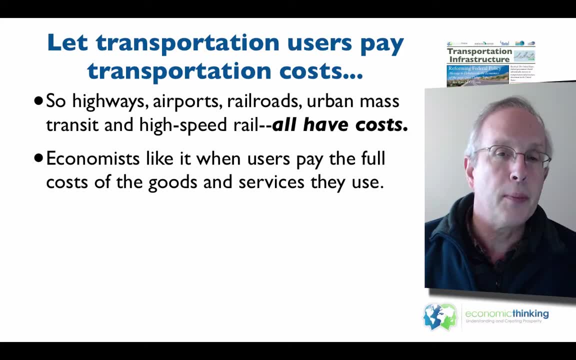 railways, airports paid for by the people who use them. All these things have costs, and economists like it when the people who use the service pay the cost. That's the way. banana technology, banana services, work in the country. Bananas are grown in Costa Rica or Brazil. 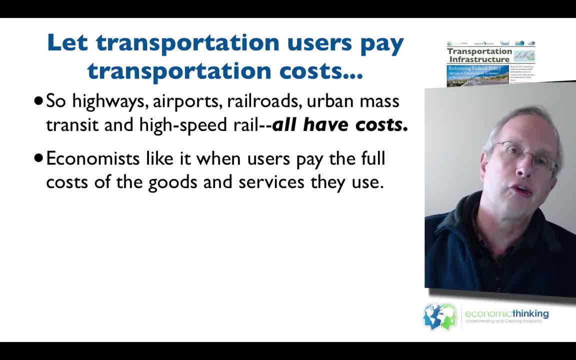 They're shipped, they're picked, they're shipped to the ports, they're loaded on boats, they're shipped to the US, they're trucked or railed to people, And that whole transportation cost for bananas is paid for by the people who use them. So that's the way economists look at transportation. 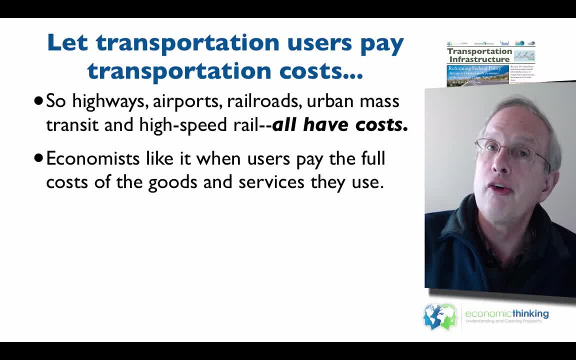 paid for by the people who consume bananas- or at least it should be. It makes sense for the people who use the good or service to pay for it. That's the just way to do it and it's the most efficient way to do it in terms of incentives in a market economy. So why not have a system where the people 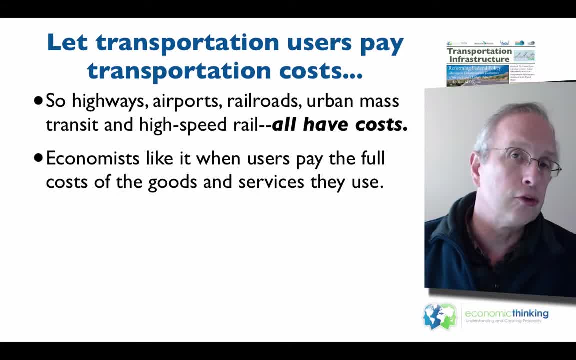 who drive on the highway pay for the highway. The people who fly in airplanes or use the airport pay for the airport. So you can have ticket fees that pay for the airport services You can have. you can have a system that pays for the airport. You can have a system that pays for the airport. 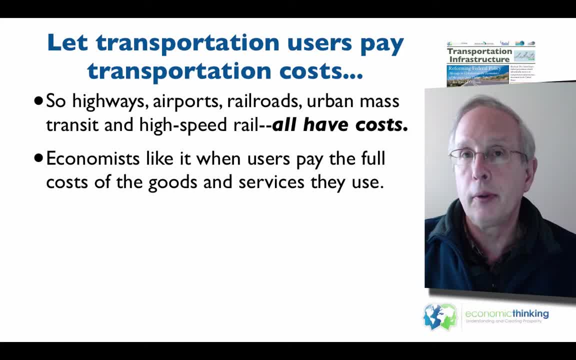 Gas taxes that pay for people. So when you buy a gallon of gas you pay a tax on that. That tax goes to pay for the highway. You can have some freeways, have tolls on them, so that people that use them pay for them, Those that, for example, can't be supported by the gas taxes. So again you're. 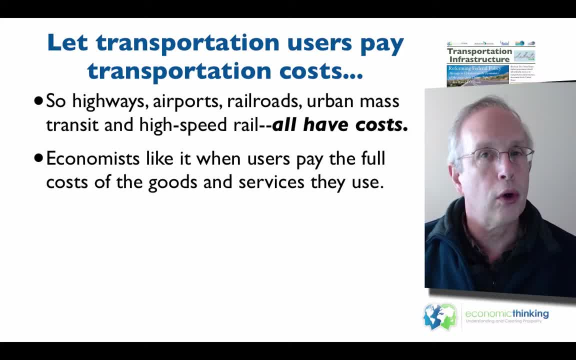 looking for an overall ideal system or a system that works as one that just makes the road system that the government runs work like private systems where the people who use it pay for it, Or at least that's the ideal. A user pay system appeals to our sense of justice and creates. 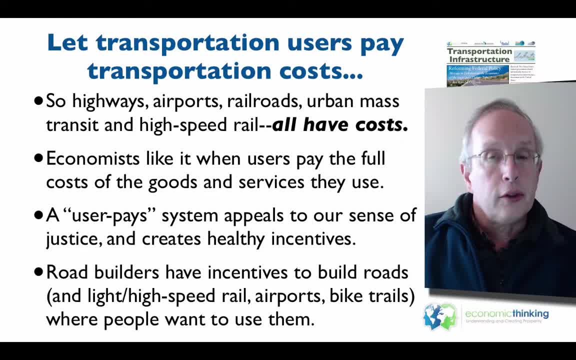 healthy incentives. Road builders under this system have an incentive to build roads where people want to use them, And the same with light rail or bicycle trails. If you have a system where the people who pay for it use it, it works better. Have I said that before? Yes, thank you Okay. 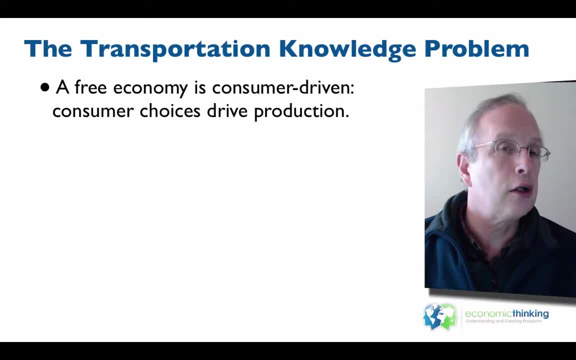 moving on. We have a transportation knowledge problem. The economy is consumer driven, The consumer choices drive production, But the producers of roads, highways, railroads don't, can't know exactly where consumers want the roads or new rail capacity or new airports. So you want, you have to have a discovery process where 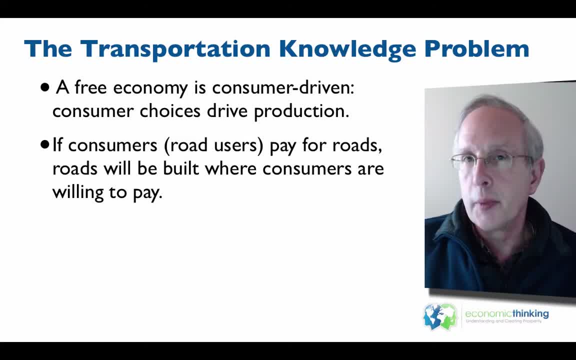 entrepreneurs are trying to figure this out. The challenge with the government- state or federal government- building these roads is that they have political motivations to do it And those may or may not be the right places to build roads. They may want to build, like a fair amount of the freeway. 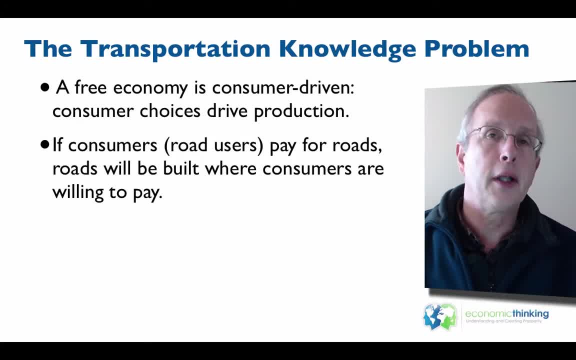 systems and airports are built where somebody with political connections owns the land, So they get the huge benefit of their land being purchased and the rest of their land being far more expensive because it's near the new highway or airport. You prefer to have a system that doesn't have those. 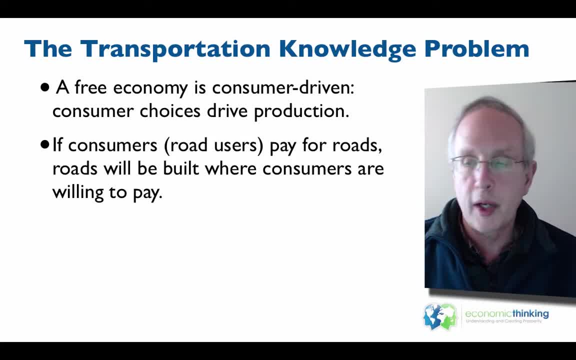 opportunities for self-dealing or corruption or whatever you might call it. Road builders have to discover where to build them And they're going to have to figure out how to build them And they will get to work. And again, that's a. that's a risk process but you'd want the people to make to take. 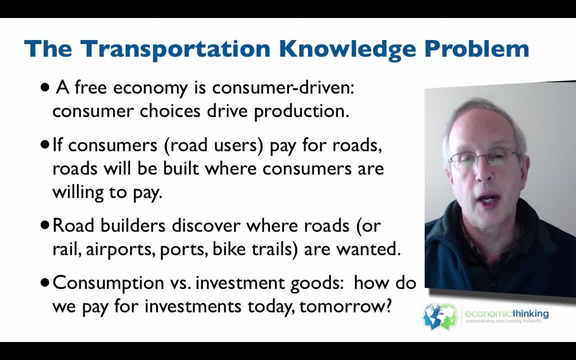 those risks who have a good incentive to put them in the right place. Another aspect of it: You can't pay for the whole highway right when you build it. Or that is to say, the value of a highway comes over the next 10,, 20,, 30,, 40,, 50 years, but the costs are incurred right now in building it. So 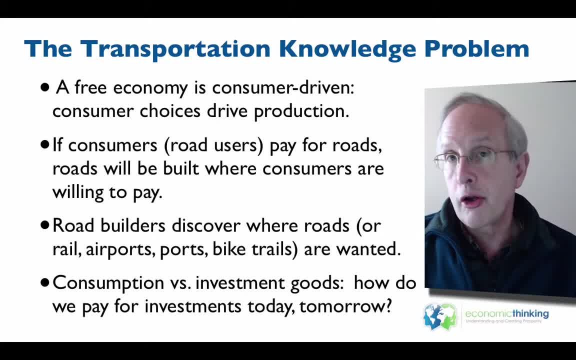 how do you finance a highway? Well, you can issue bonds that are paid for by tolls. people who use the highwayил The government sort of does it in a way that they spend the money on it and then they get revenue from gas taxes, and that's an alternative. But the idea is you've got to do the spending today, which is an investment, and pay for it in the future. 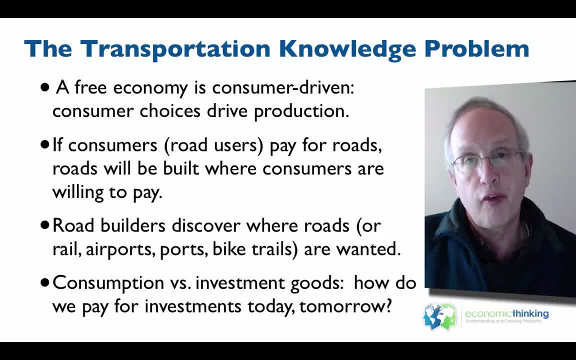 If you build it in the wrong place or the wrong kind of infrastructure, then it's not going to get paid for in the future and either the government is stuck with the road or the airport. that's unused Airports are a good example. There's empty airports around the country that are built in particular congressional districts for political reasons. They're not well used. Pennsylvania is an example for some of these. So it's a waste or a misuse of scarce taxpayers' dollars. 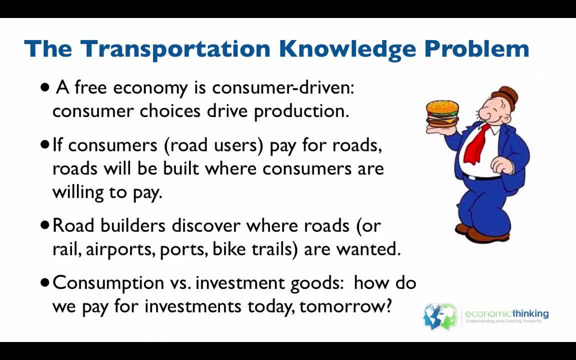 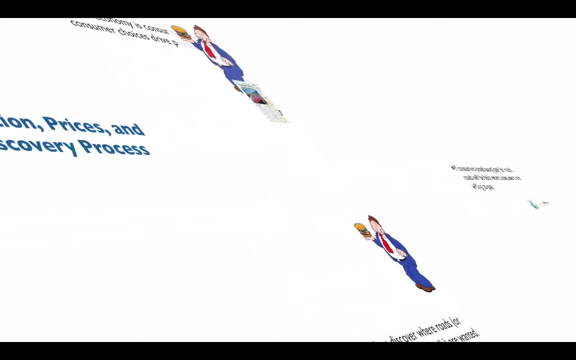 Wimpy here with his hamburger. He's more in consumer goods rather than investment goods. He is saying, as I gladly pay for a hamburger today, tomorrow and maybe slightly different hamburger on Tuesday, pay on Wednesday. In any case, you can spend money in the present by pulling assets from the future, if you invest in an asset that creates revenue. 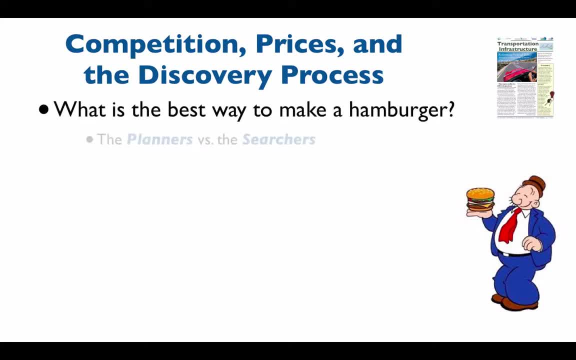 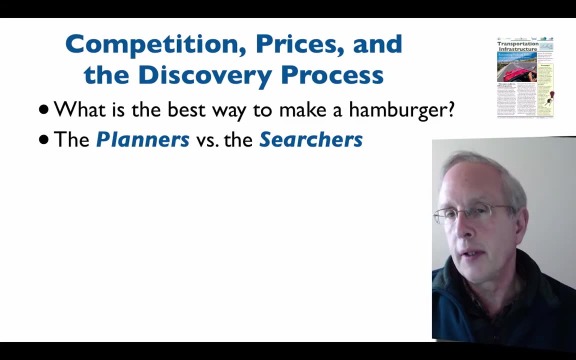 So what's the best way to make a hamburger? We don't know. Instead, we have dozens, hundreds of companies that are searching for better ways to make a hamburger. I mentioned the searching process in the sense that investors have to figure out where to build federal infrastructure and what kind to build, but there's really more options in infrastructure than just a road or a highway. 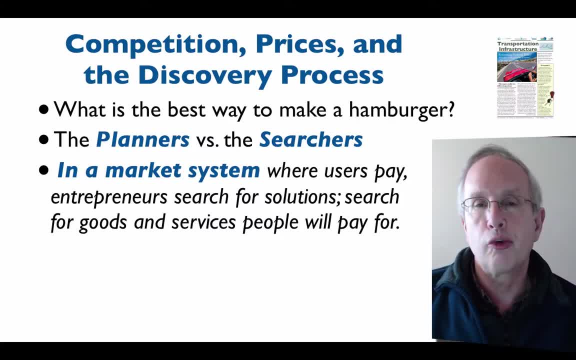 I mean, there's light rail, there's heavy rail, but there's other options as well. Entrepreneurs are searching for solutions For goods and services people are going to pay for. So we want entrepreneurs to innovate, to find new ways to use assets more efficiently. 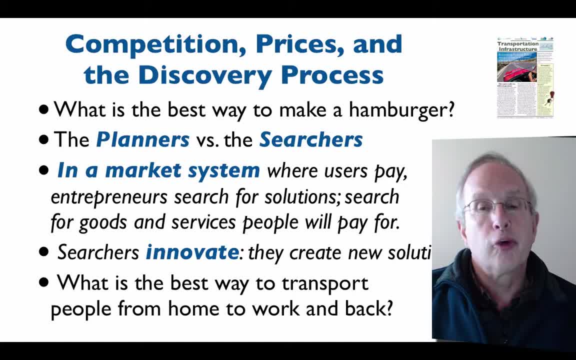 So if your question is: what's the best way to transport people from home to work and back? Well, roads do that now, or light rail can do that, or subways. However, what if that's the wrong question? What if you can transport people via electrons to work? 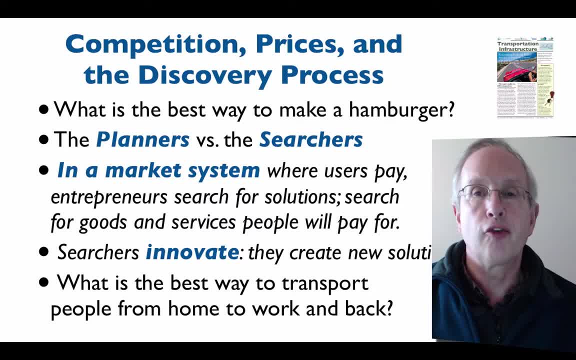 Not a transporter, but what if you've got a light rail? Well, you've got a Skype video conference, where people at home are in an office, where they can be seen by video or a three-dimensional hologram. So you don't know if the person's actually sitting in his office or not until you swipe your hand through them. 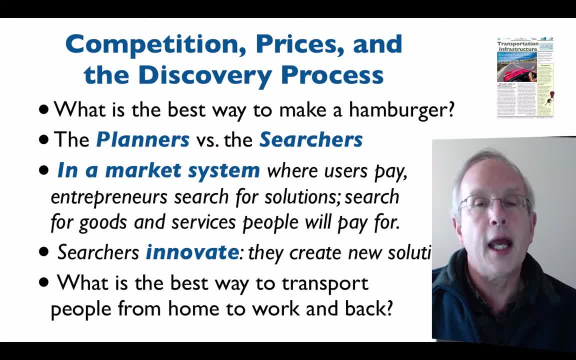 And if they're there, of course, you've whacked them. In any case, we want to look for new ways to solve the transportation problem, but, for example, in shipping goods and getting people to work, there's many, many options that people don't often discuss. So let's look at the cost of congestion first: Some $200 billion wasted annually in transportation delays for freight. The picture on the right is one from China, as the trucks are jammed up waiting to get to port. The one on the left is a highway in the United States, jammed up at rush hour. This is a lot of money wasted on this, So let's look at how you can fund new roads again without a net cost. Some $70 billion of fuel are wasted each year as cars are stopping and going at 5,, 10,, 15, 20 miles an hour, instead of going at 55 or 60. 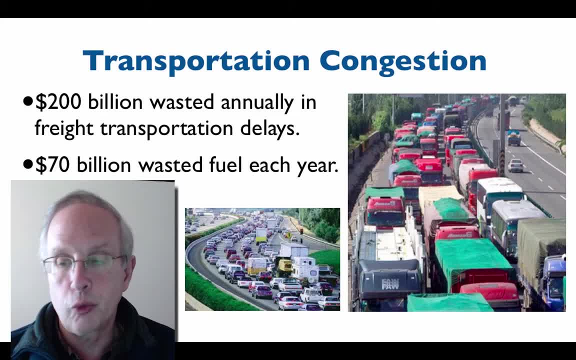 That stopping and going is wear and tear on the cars and is wasting fuel. So by fixing the system so it works, you can save $270 billion simply by having freeways that are properly managed. So it's true, it costs money to build new highway capacity. 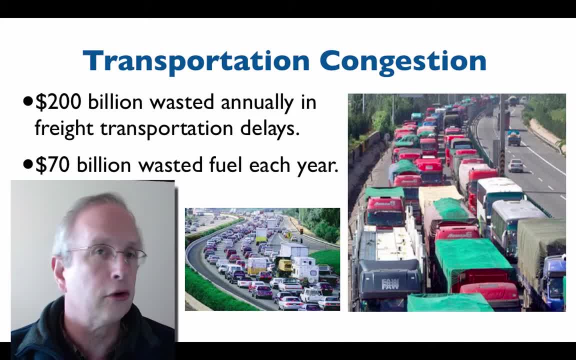 but here's $270 billion a year that are available to fund that increase in capacity or increase in technology that improves management. What's the best solution to this? Well, a challenge is for the affirmative. you're sort of pretending in debate that you're the congressman offering the solution to the world. 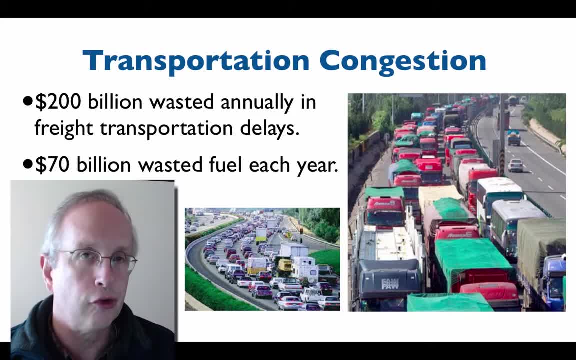 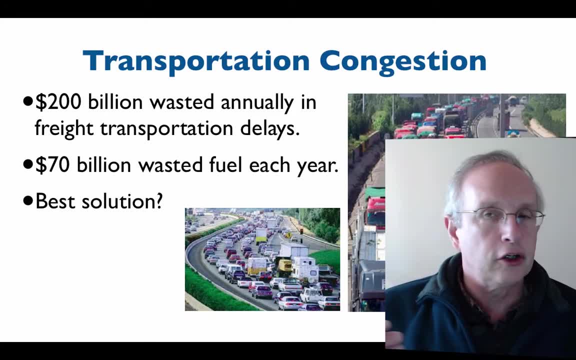 but in fact, you can't know the solution. Congress doesn't know the solution, Nobody knows the solution. Instead, the solution is one that's discovered, that emerges through the interaction of hundreds, thousands of entrepreneurs with ideas and investments, millions of customers, transport, people making decisions about where they want to go and how they're going to adjust their lives. 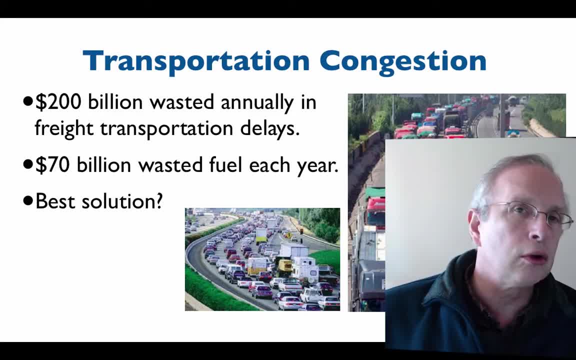 shipping, people, purchasing agents. That whole adjustment process is managed throughout the economy on the basis of prices and markets. Because prices communicate information between people buying services, people producing them, In transportation, we've got a problem: We don't have flexible prices. 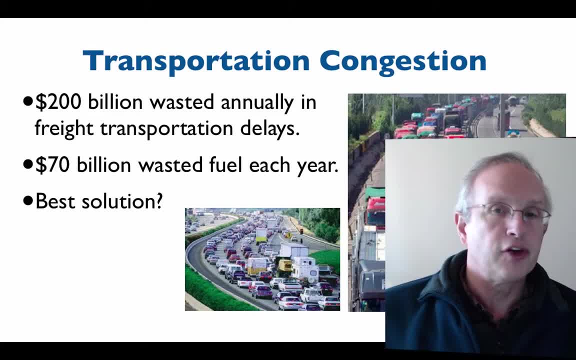 Highways are free. That's why they're jammed at rush hour every day. If you had a way to adjust prices, a way to use prices to communicate information, you could better deal with this. So again, the planners versus the searchers. 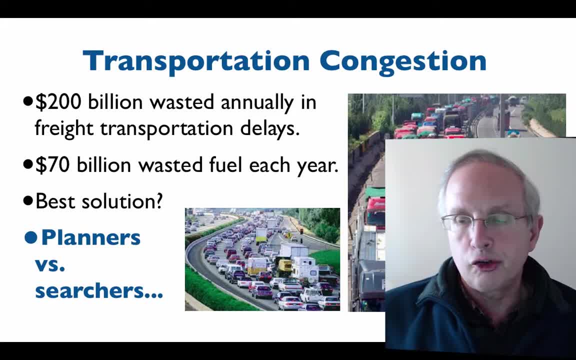 William Easterly uses this model In his book White Man's Burden. it's discussing the problems of foreign aid, Market economies and market sectors of the US economy. have searchers trying to solve problems? The computer industry, tech industry, TV industry? 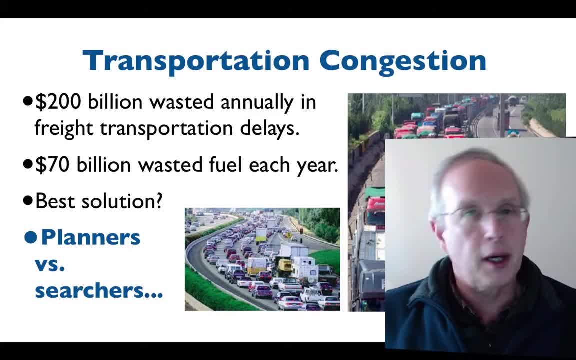 But we also have sections that are top-down planned by federal transportation agencies, the Department of Transportation, state agencies. These city, state and federal agencies are trying to plan from the top down how to solve transportation congestion, But they don't have access to the information that would allow those solutions to emerge. 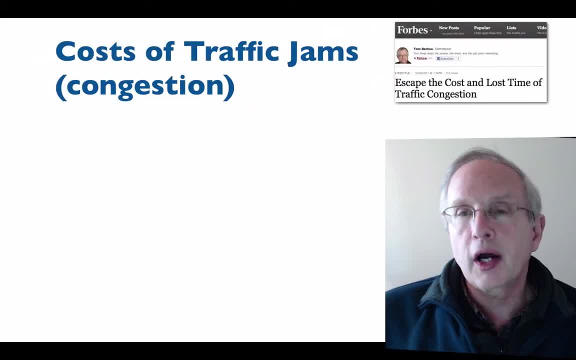 This is the ideas that Friedrich Hayek talks about in Use of Knowledge in Society And Leonard Reed discusses in his book I Pencil, And I'll maybe have a separate box to discuss that. Now let's talk about where the money can come from. 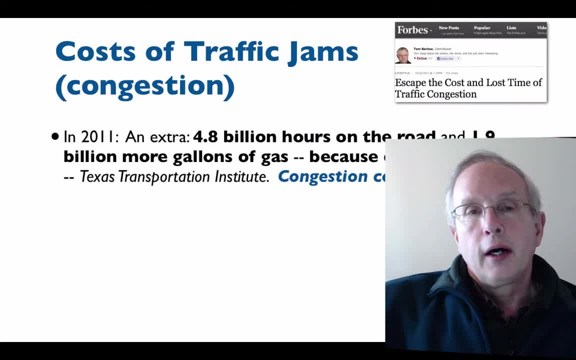 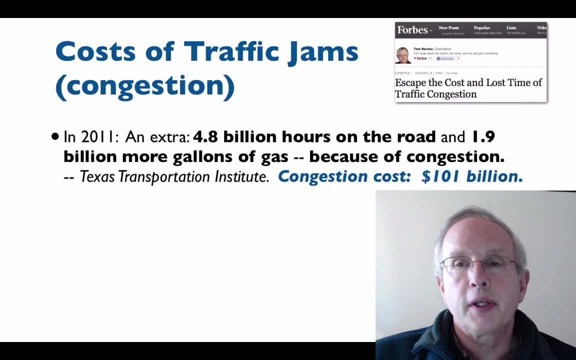 I mentioned the hours and time wasted: 2011,. an extra 4.1 billion hours on the road. according to transportation economists- Texas Transportation Institute- 1.9 billion more gallons of gas because of congestion. So congestion costs in this measure, $101 billion. 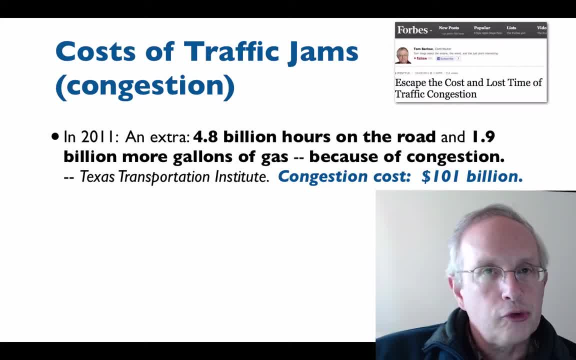 If you think about this in terms of traffic jams. I met a fellow who lives in Federal Way. He commuted to Linwood every day For his work. it was an hour each day each way, So he spent two hours on the road. 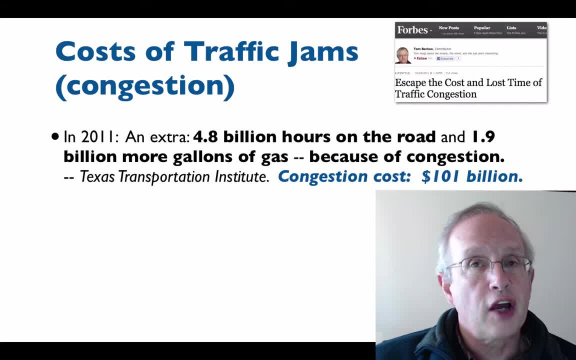 One hour of that was congestion. That is to say, if the freeways worked going at 45 to 60 miles an hour, he would have got to work in a half hour, would have got home in a half hour Instead, because so many people are on the highway at the same time. 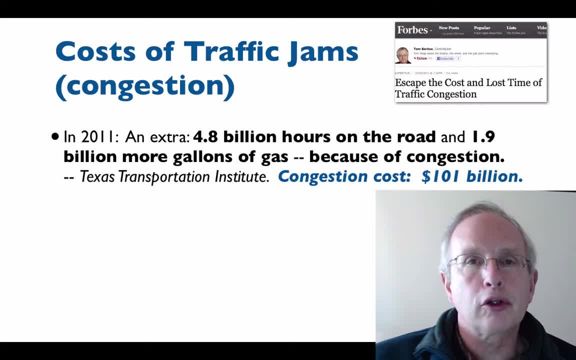 he's an hour getting to work, an hour back, So that's an hour lost every day And he's stuck in traffic Plus the gas with stop-and-go traffic. Now if you think about the proposal that says: OK, we're going to put a toll on the freeway and charge everyone $5. 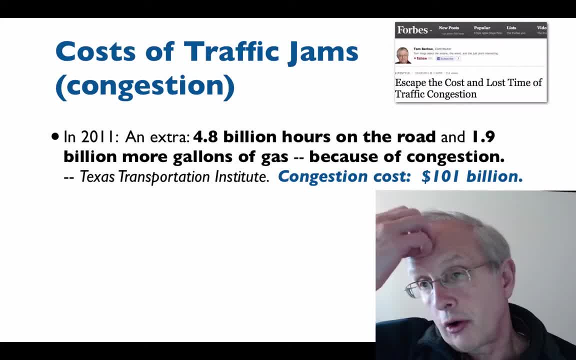 to drive to work in the morning and $5 to drive home. So that would seem to cost him an extra. you know $10 a day. But if through paying that he was able to go full speed home and back. 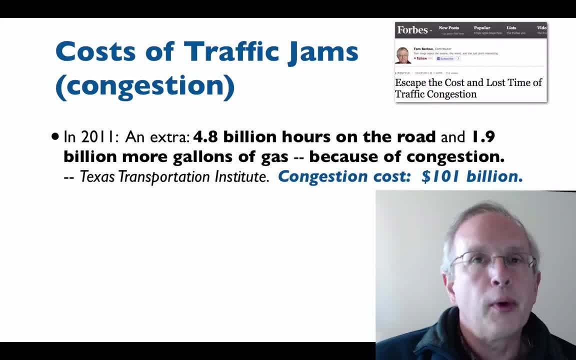 he would save an hour. So this guy was a Boeing engineer. He would save an hour of time and pay $10 to do it. That's a tremendous deal for him, right? Because his time is working for Boeing, He gets paid far more than $10 an hour. 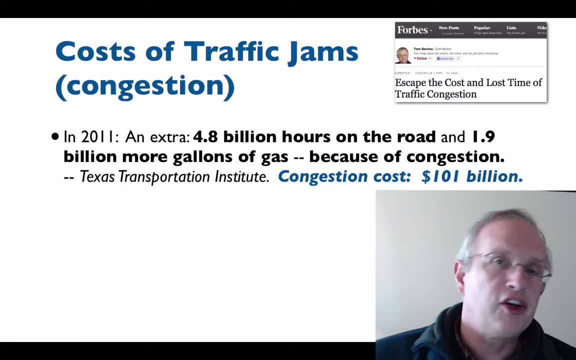 He values his leisure at more than $10 an hour. If he had the option to pay that, he would, As would millions of other Americans. So, in a sense, every day that there's a traffic jam, these are people who would be willing to pay money to get to work or to get home at rush hour. 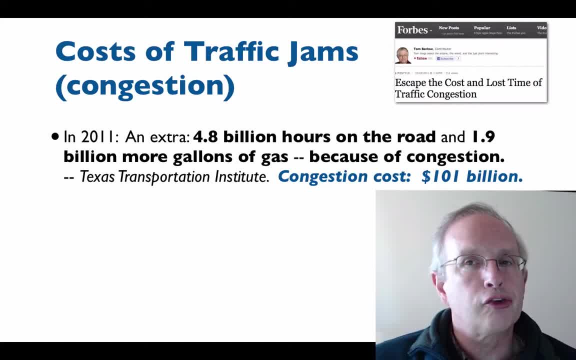 But they're not allowed to because we don't have a system that allows prices to handle the demand for the product so that it's used efficiently. We have prices at the movie theater right. More people want to go to the movies at Friday night and Saturday night. 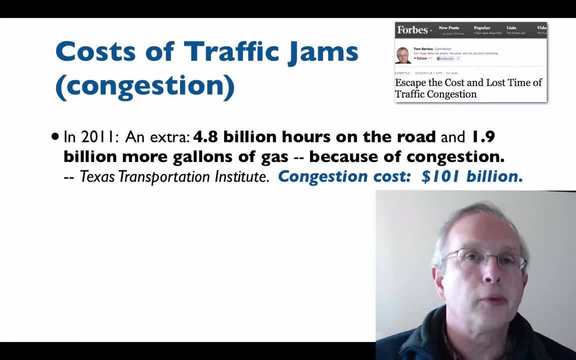 So how do theaters handle the fact that they've got scarce number of seats in their theater? Well, they charge higher prices People that go to the matinees on the weekdays and the afternoons they pay significantly less. So the movie theater is dealing with a problem. 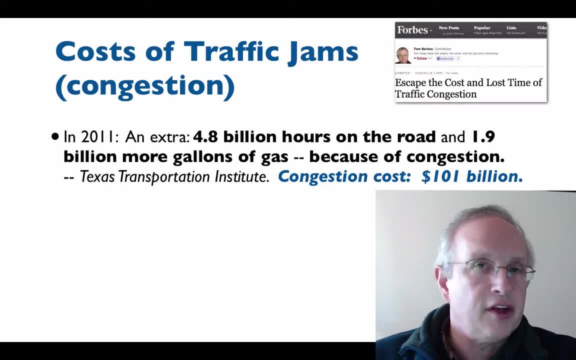 that, though most people want to go to the movies in the evenings, there's only so many theater seats available, So they raise the prices at that time and they lower them at other times when people are less likely to want to go. But many people can change their plans. 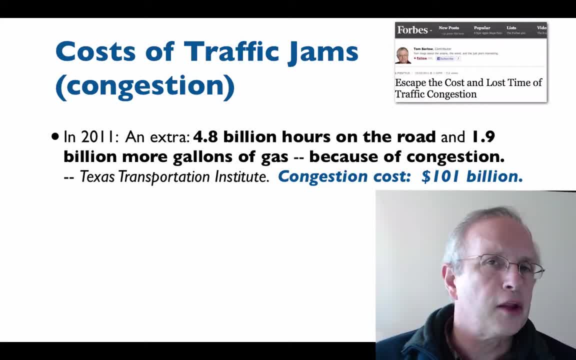 Similarly with the highway: 50%- 40% of the people that are on the highway at rush hour aren't going to work. They're on the highway for other reasons. There are lots of people that can change their driving patterns without great cost. 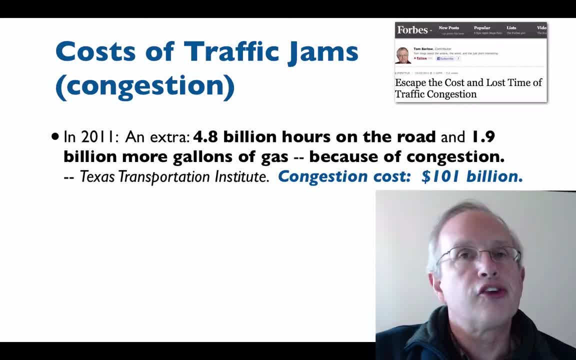 If there was incentive to do that. Charging people to use the freeway when it's most valued is one way to do that, And that's a big debate on that. This is a discussion over congestion pricing, And the argument is that you could reduce congestion delays. 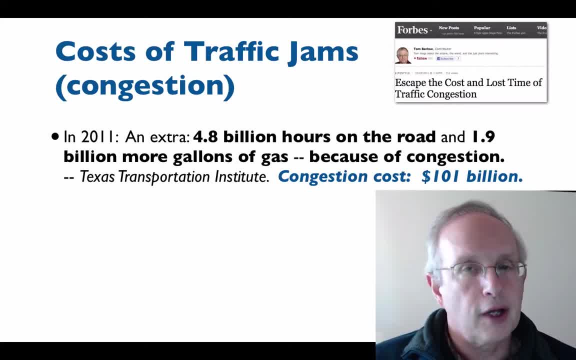 save hundreds of millions, billions of dollars a year, have more money to put in to expand infrastructure, simply by putting a price on peak traffic time on the highway. Population's gone up by some 80 million since 1982.. A lot more cars- some 124 million more cars on the highway. 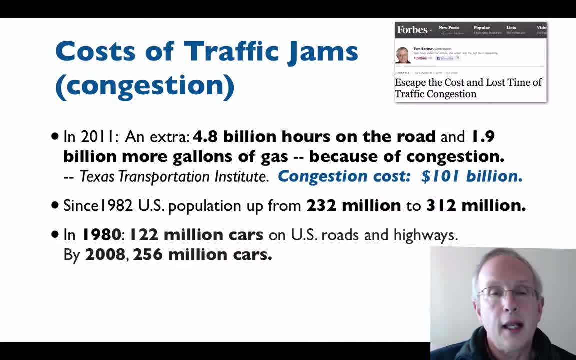 than there used to be in 1980 to 2008.. So the question we ask is: has highway construction expanded to keep pace with the increase in highway customers, Or has light rail or subway expanded to keep pace with the increased population? And the answer is no. 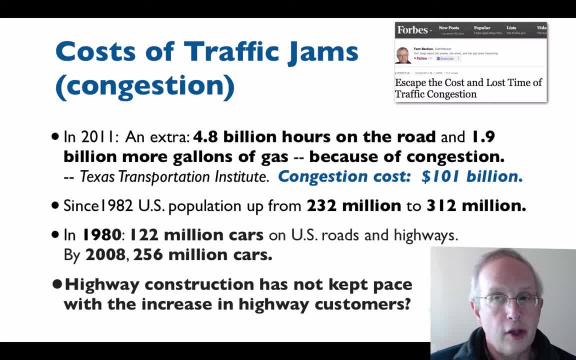 This has to do with a number of demographic changes. That is, the suburban population no longer commutes to the city for jobs each morning. Instead, most of the commutes in Los Angeles, Seattle, most cities, most western cities and southern cities are from an edge to another edge. 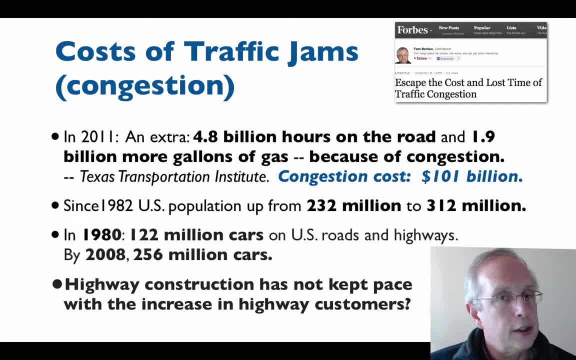 So they're going around the loops in the towns. They're not going from the outside to the center, which is why light rail and heavy rail and subway aren't efficient. They're efficient ways to deal with transportation because people are spread out in the way they work. 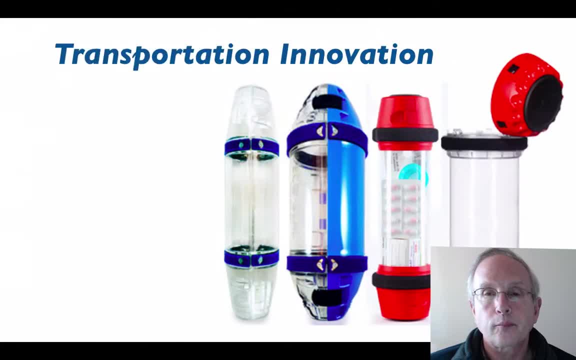 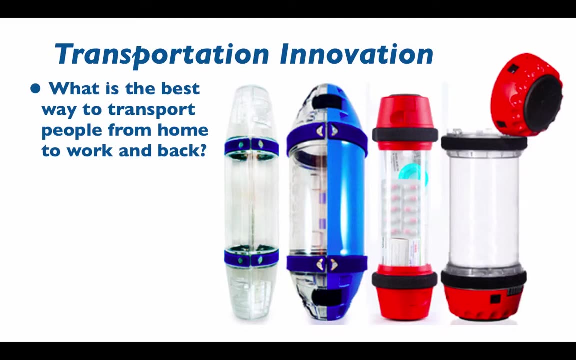 Anyway, more to that debate, but that's a brief note on it. So are there alternatives to the current status quo in terms of transportation? Well, here's some transportation alternatives. You may not know what those are right off When we ask the question how to get people and goods and services. 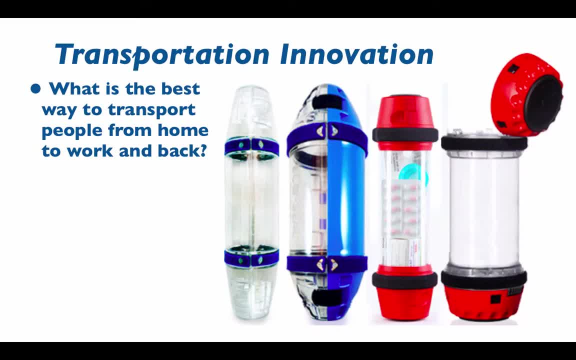 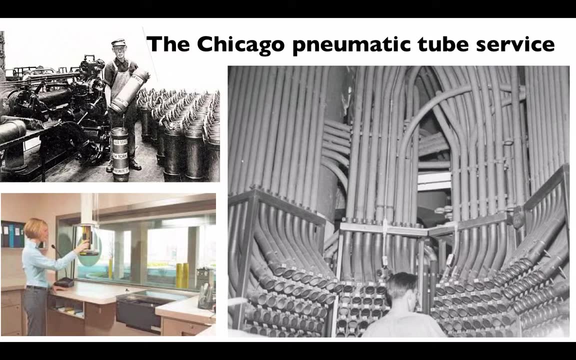 from where they are produced to where they're wanted. I mentioned meetings, teleconferencing, but maybe you could also send goods and people through pneumatic tubes. That's what Chicago used to do. Chicago had a system of pneumatic tubes that connected the downtown buildings. 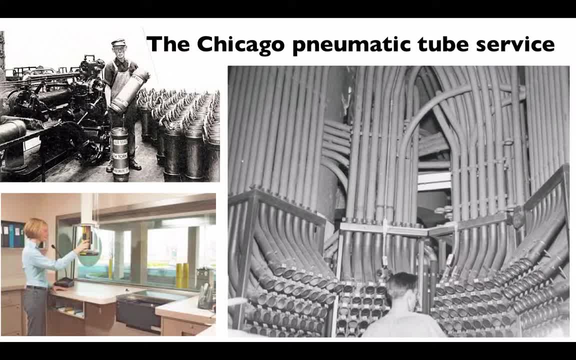 and people in any building could send a letter or a package to any other by putting it in a tube and it would zip along to another place, And this was before computers. This was with mechanical systems that were not efficient by our standards. You still see these in banks and a few other areas. 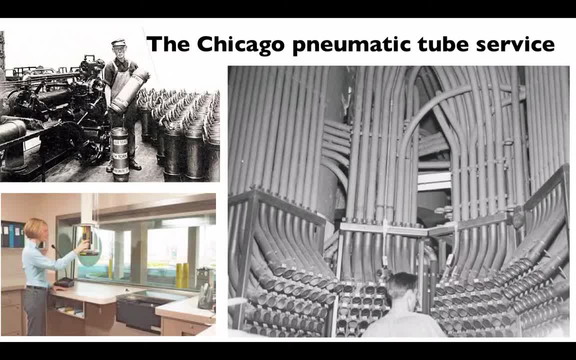 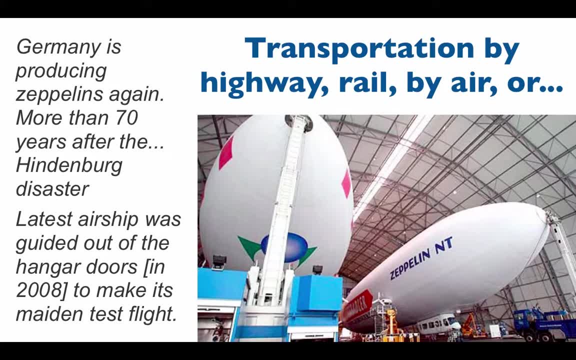 where people's deposit goes through, sort of a vacuum tube. But that technology is available and could work in many ways. I'll come back to that. What about shipping things by rail and freeway? We've got trucks shipping stuff all over. Why not use Zeppelins instead? 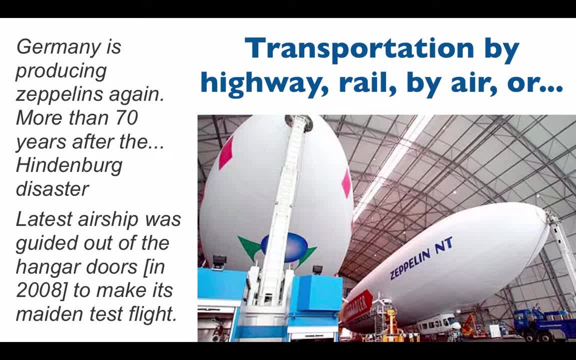 These are filled with helium. The technology is much more advanced- We see the Goodyear blimp advertising- but Zeppelins could also be used. They could also do a lot more to transport goods and services. Maybe you could even have buses run elevated. 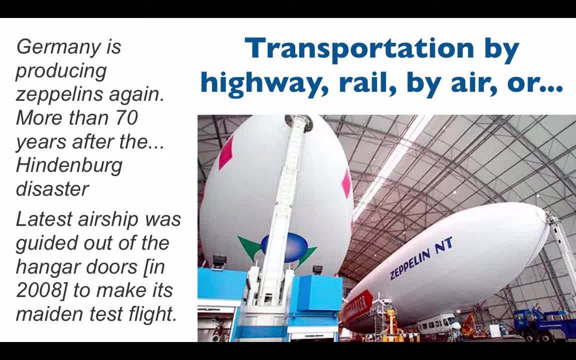 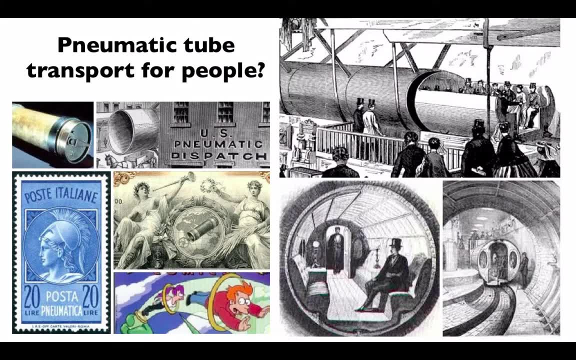 There's more to that story. The great story of the R-100 and R-101 debate on travel is fascinating, But for here I just mentioned that Zeppelins are. I'm sure some students will be interested in the Zeppelin affirmative. 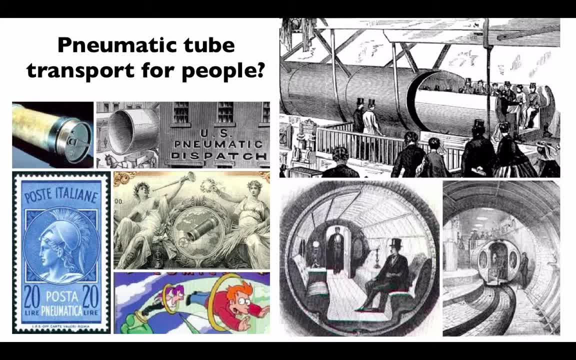 for transportation infrastructure Pneumatic tubes. The London tube was the transportation system for sending people around London. Basically, you're building a tunnel, a tube, and sending people along it. To what extent could that technology be revived and modernized in the computer world? 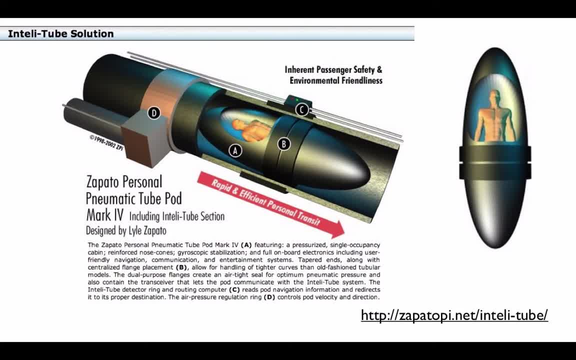 If you think about the modern light rail systems- the New York subway- most of that technology is 100 years old. These are heavy systems that are less than ideal. Here's Zapata. This is a personal pneumatic tube pod that allows people to travel around the city. 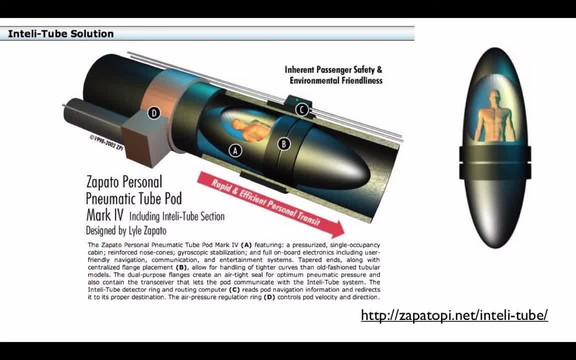 Apparently, you have to take your clothes off to travel in this, But the idea is you're zipping around a vacuum tube. It's got information computers on it to move quickly- much less power involved- And so the question is: how expensive would it be to build this kind of infrastructure? 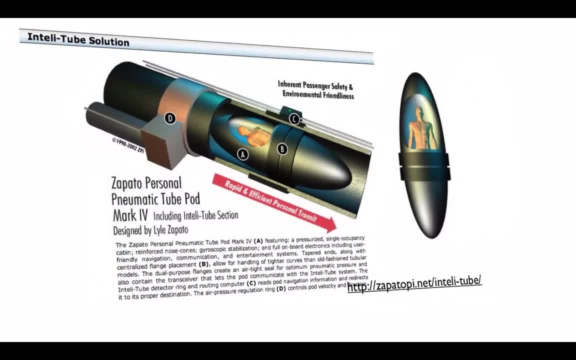 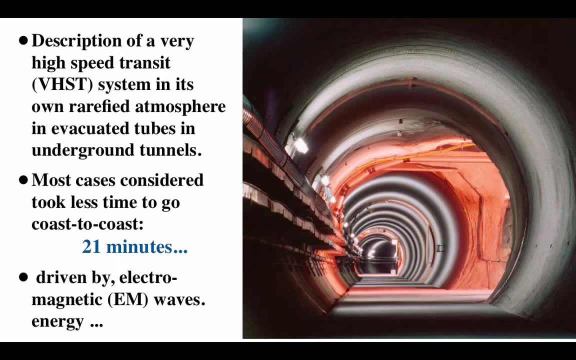 compared to building more light rail or freeways or airports. Students that have looked at these issues before have looked at high-speed vacuum tubes for long-distance travel. Gerard K O'Neill at Princeton developed this technology, at least the ideas of it, many years ago. 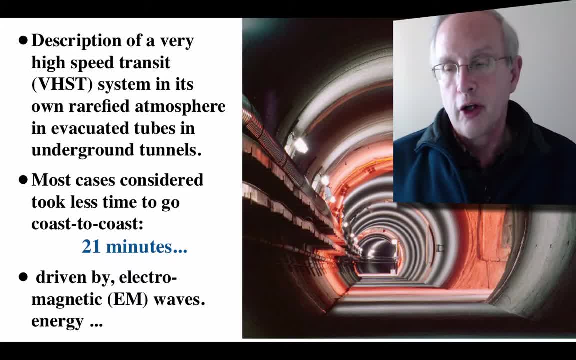 But basically it's 21 minutes to go from New York to Los Angeles through a vacuum pneumatic tube. It'd be expensive to build, expensive to maintain, but you could send people rapidly and accelerate them smoothly so that they wouldn't be flattened like a pancake. 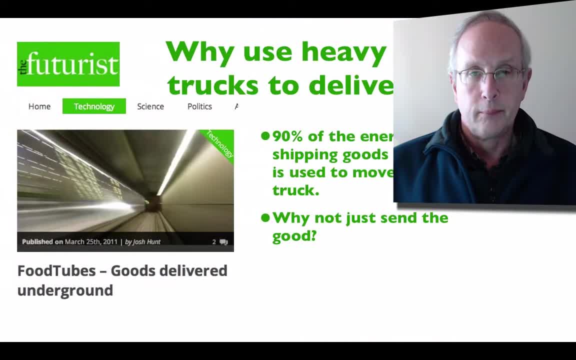 but get them from one place to another rapidly. This company Article in the Futurist says: why use heavy cars and trucks to deliver goods? 90% of the energy is accelerating and breaking the truck and the car. Why not send goods through food tubes? 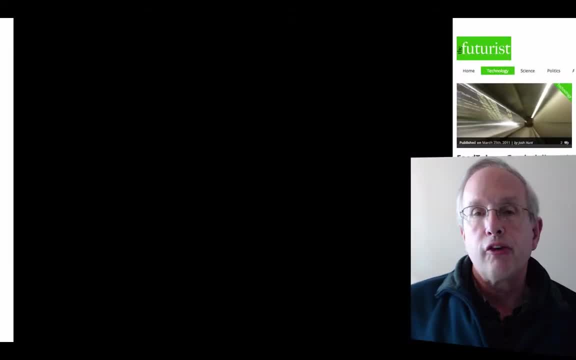 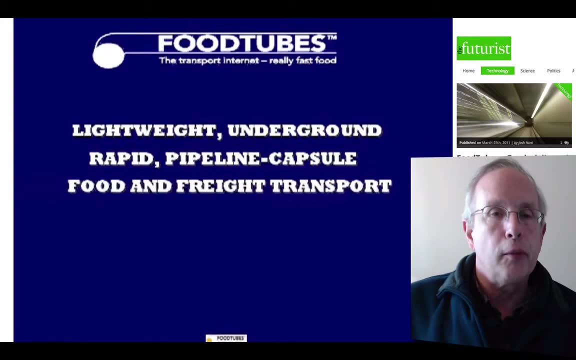 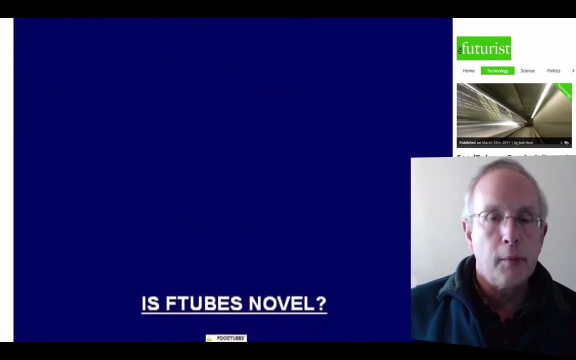 through vacuum tubes underground. You can find this on their website. This is a little inexpensive video deal. the animation that just shows their system. This is mainly an environmental group claiming: look, this is going to reduce CO2 emissions, and so forth. 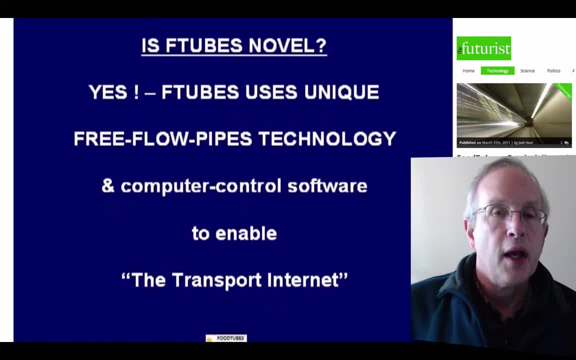 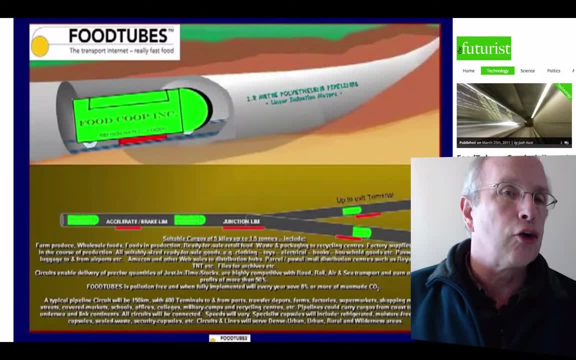 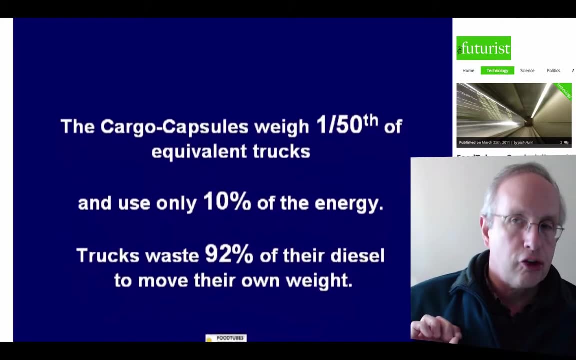 And whether that's a big deal I can't say. But the idea is these tubes it's much less expensive to tunnel than it used to be If you look at the incredible advances that the shale gas drilling has done. it's lowered the cost of rapidly drilling small tunnels dramatically. 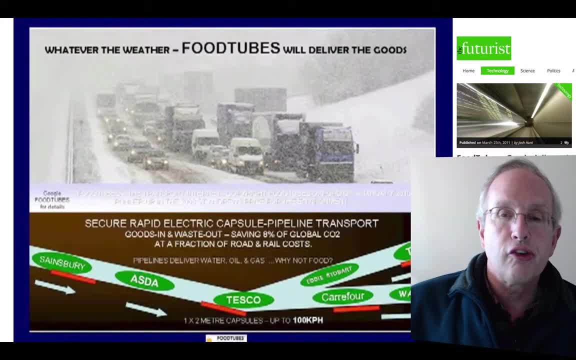 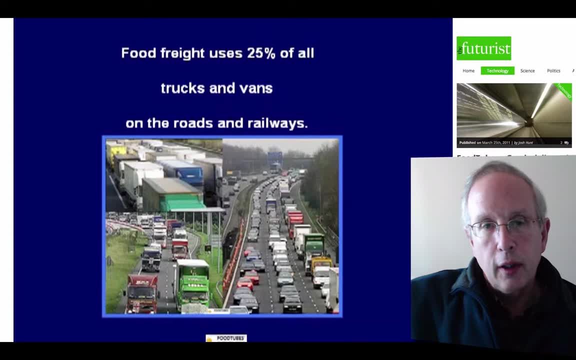 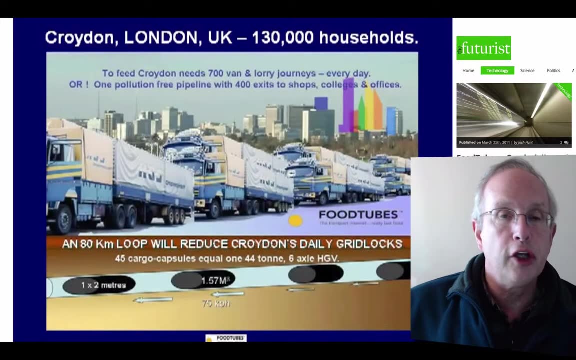 just in the last 10 years. Maybe this horizontal drilling technology could be used for drilling tubes that are filled out with these vacuum tubes and then, instead of having all these trucks on the highway, goods can be delivered quickly from one part of the city to another. 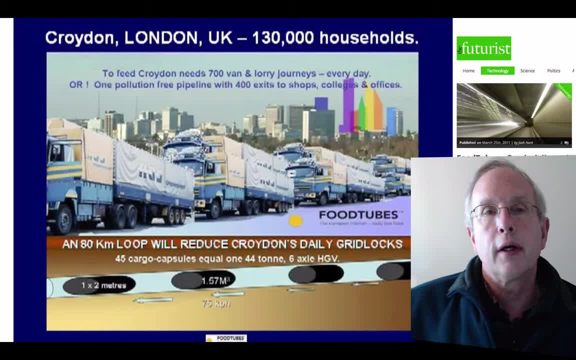 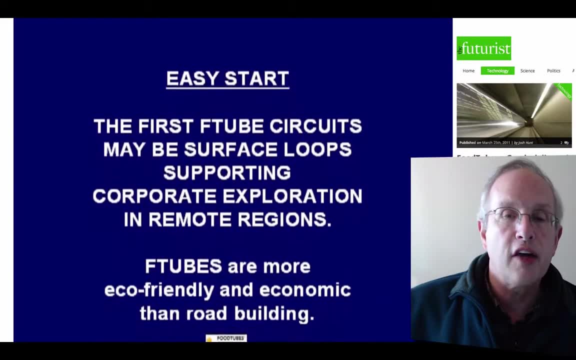 So this is a proposal for one section. in part of London, 130 households could be connected with these tubes, they argue, and save money, save energy and so forth. Is this a good idea? Who knows? You'd rather have investors.